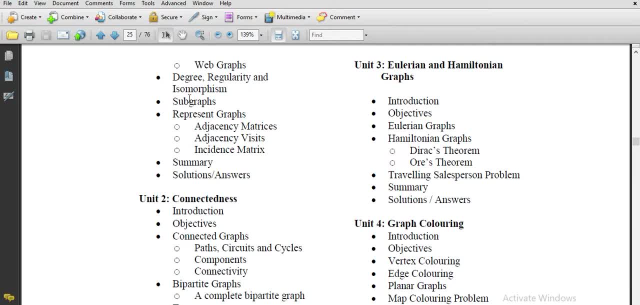 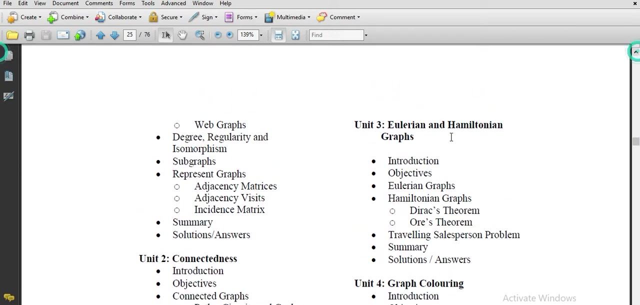 and lists also the isomorphism. So in this I will discuss about this connectedness, in which I will discuss about the paths, circuits and cycles. What are the differences between these? and I have already completed bipartite and complete bipartite Right, and then I will cover this Euler and Hamiltonian graphs: right, this unit 3, right, And before that I have already covered 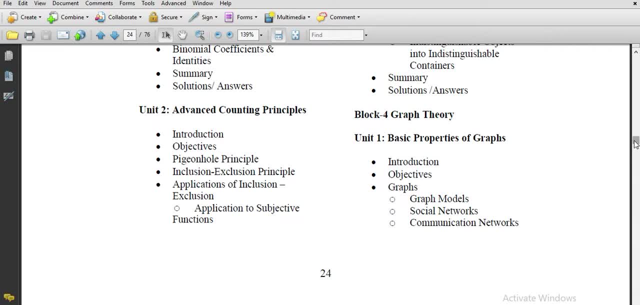 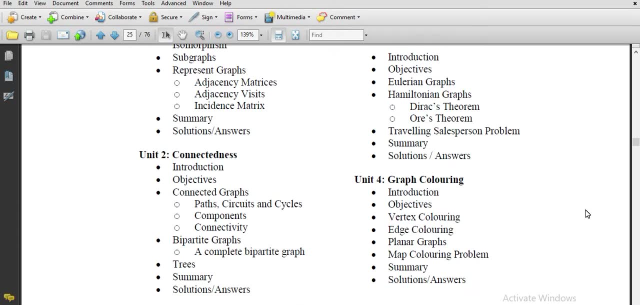 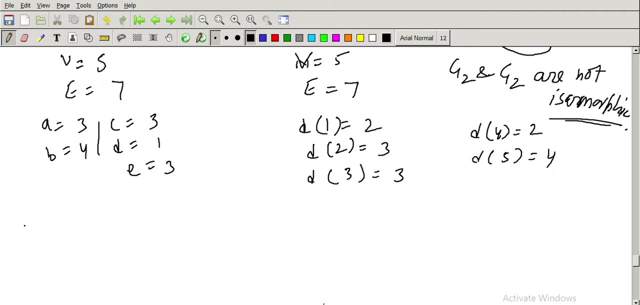 the basic properties of graphs, in which I have discussed about the various types of graphs, and all right, So let's start this right. So I will start from the topic of where I have left- isomorphic and complete bipartite, And after that. so I begin with this. circuit, right. What path? So, first of all, what is the path? So path is a sequence of ages, right. What is the path? is the sequence of ages right. So path is the sequence of ages right. So what is the path? is the sequence of ages right. So part of a path is the sequence of ages right. So that means you can write the bottom line or the kinematics here: what is the quantity of ages? So? what is the path? So the line plus or minus. so this will be used as it bra, then that will be called the었다 climb. so there will be a다 вари here of alpha, then there will be a der subject and theata. okay, Now we're going to shocking with the pathNow to what is the path of ages? So path is the sequence of ages, right. So here we have the path, sum series. don't write down anything. mis jurisdictions can be taken here, because grammar is the judges at the center of empiric in this language. 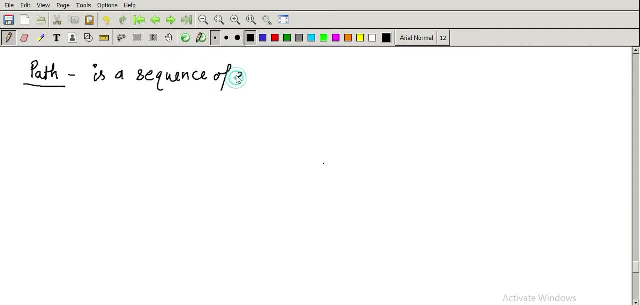 the sequence of edges is a sequence of edges that begins. that begins the begins at a vertex of a graph, at a vertex of a graph. you know what is a vertex? it is a, basically a node, right, okay? graph and travels from and travels from vertex to vertex. 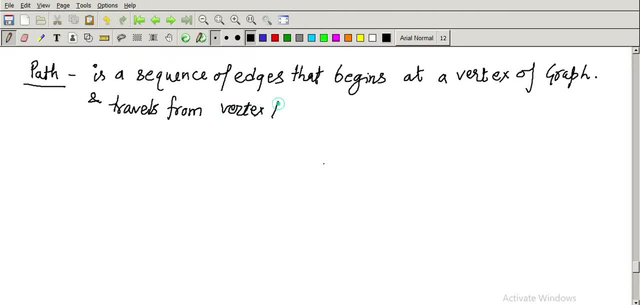 vertex to vertex, along the edges of the graph, along along the edges of the graph, right the edges of the graph. sorry. so here I I have this right example for you. let's understand by this example that I have this example. this is your graph, right? this is a graph because it has edges and vertices, and 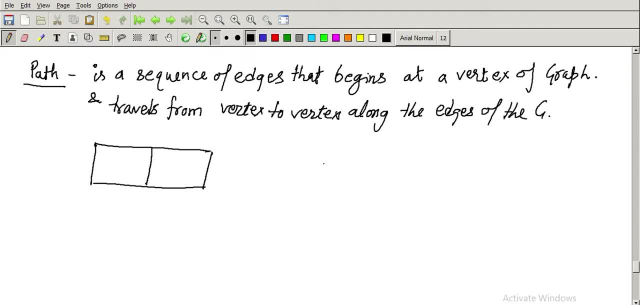 this is like right. so this is this vertex is connected to this right. this is your avertex. this is your B, this is C, this is D, this is F and this vertex is F. So B is connected to F and D is connected to C, right, In that way, D is connected to C. So this is a graph. 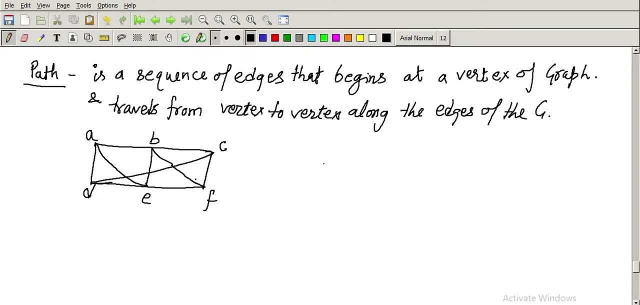 right. Very simple graph, right. So if I need to find a path of length 4, right, A path of length 4, right, Between A to E, right Between A to E, A to E will be A to B right, A to B, then B to C, then C to F, then F to right. So this, if I use, 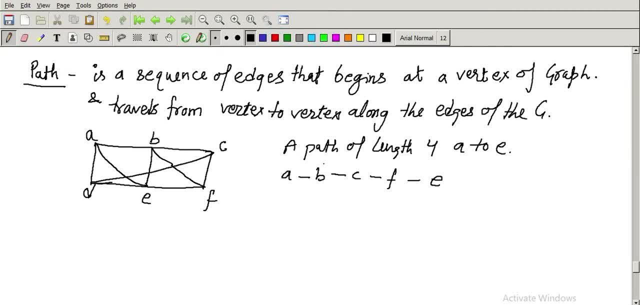 this color. I don't know what's happening here. Okay, no problem. Okay, So here I can. okay, I use like this direction: So A to B, right, A to B, then I go B to C, then I go to C to F, then I go to F to E. This is of length. 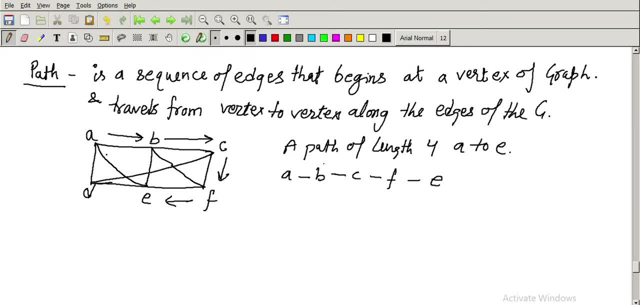 4. I can also go directly from A to E by covering only this one edge. So this is because they have asked of length 4.. So this is one. Length means the distance between the two adjacent vertex is means that there is one. 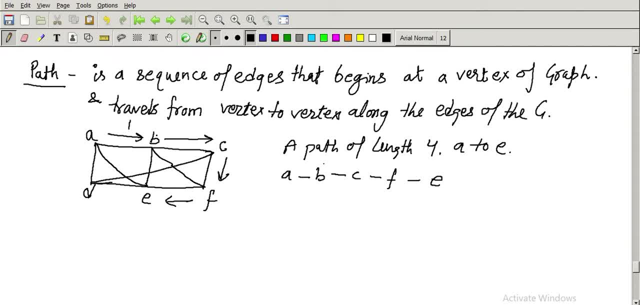 unit. so one step, right. So this is one, this is the second step, okay, And this is the third step and the fourth. So that's why this length path is 4.. So from A to E. 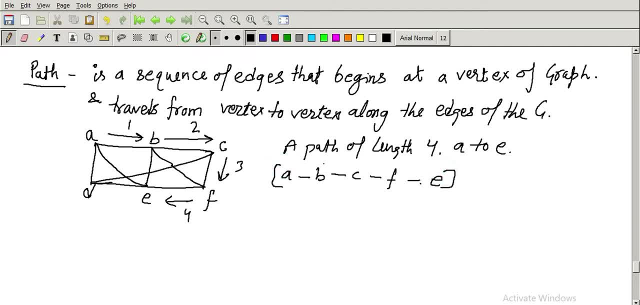 we go like this, in this way, Right, Okay, So this is a simple path. Why is the simple path? Because there are- these are the edges between these when we travel from A to E. there are edges, Okay, So consider. 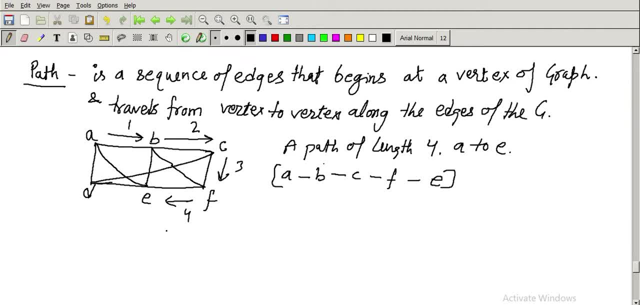 this another path. okay, The path is D. Okay, let me write from this side. right, That was your 4.. So let me write here: this is D, E, C, okay, A, If I write this. so this is not a path. 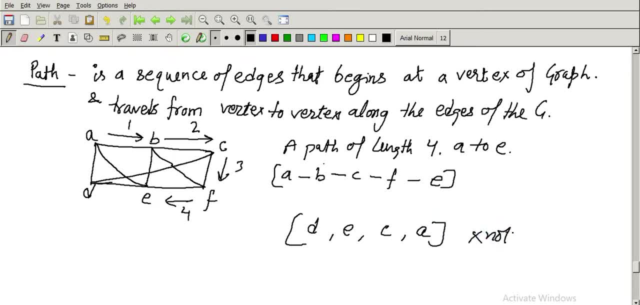 right, This is not a path, Not a path. Why it's not a path? Because when we move from D, you are here, Wow, moving towards e. yes, that's okay when you're moving e to c, e to c, so i don't have any direct. 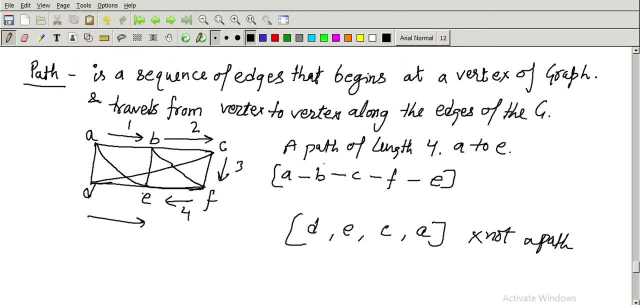 path from e to c, because if i want to go from e to c i have two ways: from e to b and then b to c, and then the second is e to f, then f to c. so there is no direct is, but they are saying that they have. 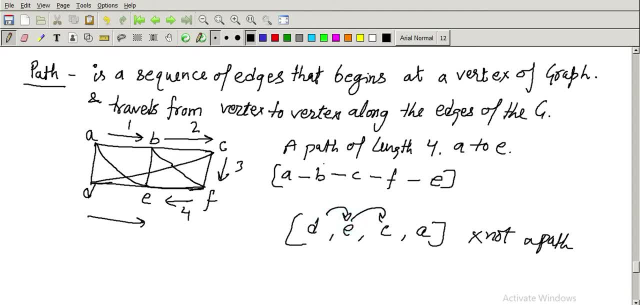 gone as like d to e, then e to c and then c to a. so because it's, it's not a path, because there is no edges. there is no edges between, there is no edges between e to c, so that's why it's not a path. 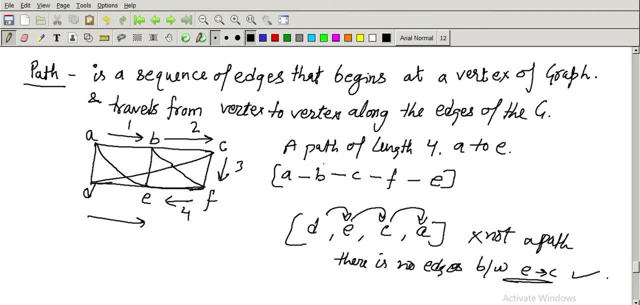 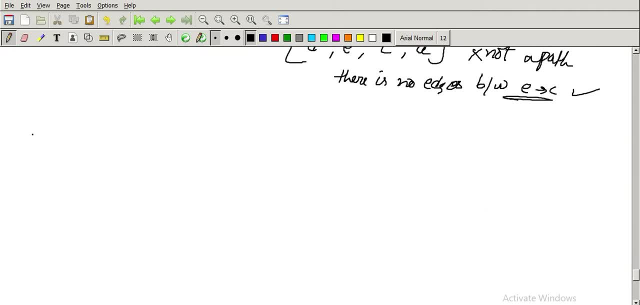 it's just for your example, and please do remember this concept of path, right? because when we, um, when i talk about the eiler path and hamiltonian path and hamiltonian, either uh circuit and hamiltonian circuit, we we must remember these small concepts: or simple path, or the circuit, or 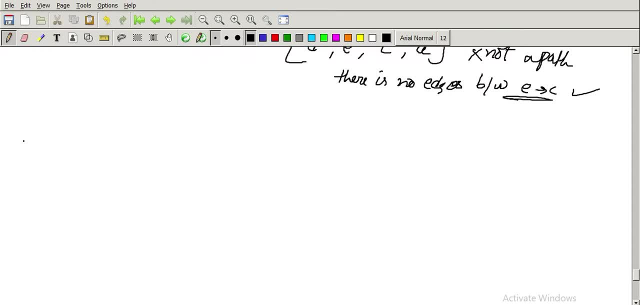 right, simple graph and multi-graph and all. so once you know that these concepts, you will be right, you will be, uh, it will be easy for you to graph those concepts right. so here the connected components. when I talk about the connected components, sometimes we have the different components, like this is: 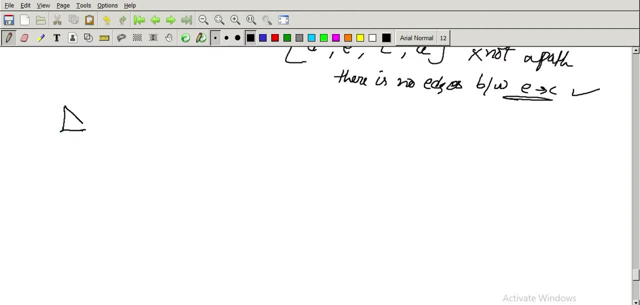 like, here I have this component like ABC, right, and here I have another component of this ground which is like this: okay, right, D, E. so this is a graph. okay, this is a graph. this is a graph, but it has two components. these components are not connected to each other, but this is a graph. okay, this is a graph. G having 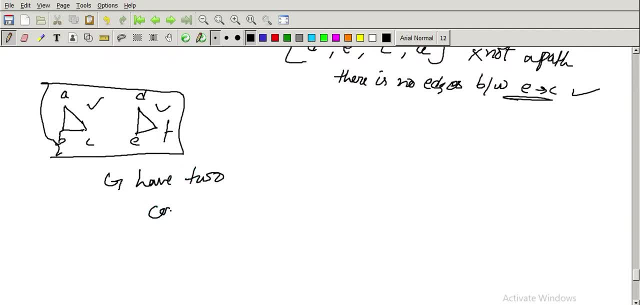 two components, right, but these are not connected to each other. okay, so, likewise, this is the concept of components of of a graph, right, so we have these types of graphs also. so we have these types of graphs also when, right now, I talk about your circuit, right, so a circuit is like this, in this, 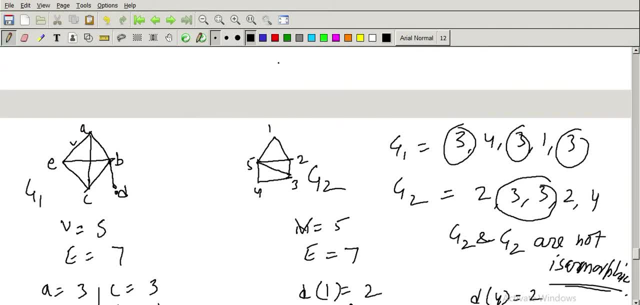 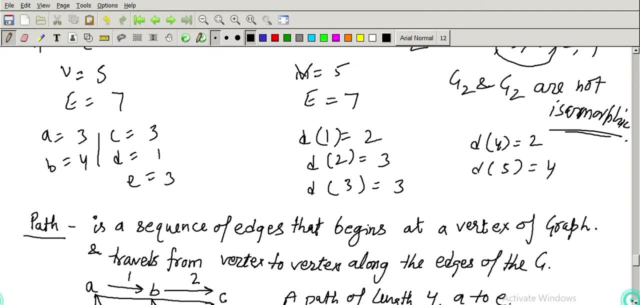 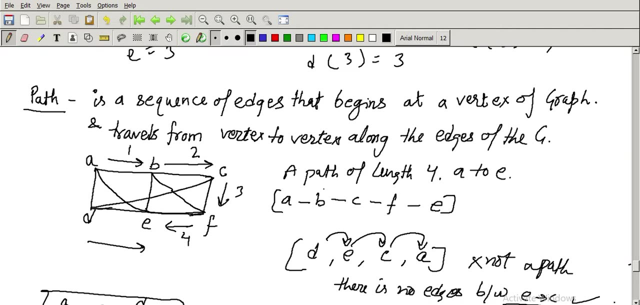 example- this previous example- we have a circuit right. circuit means circuit cycle, right. so what is what do you mean by a circuit right? so part is that the a CyS for all the vertices, vertices. so when we start from a vertex and go to another vertex, there must been as between these. 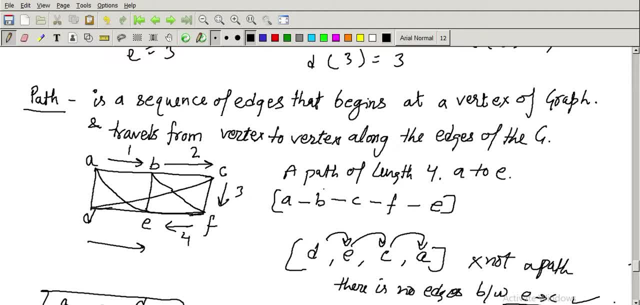 two vertices. so we we say that yeah, there is a part. so if there is a specific path or if there is that path, if I start from A here and travelled through these all the vertices and I end on A, then it will be like your circuit, right. ok, now we understand the concept of Euler. 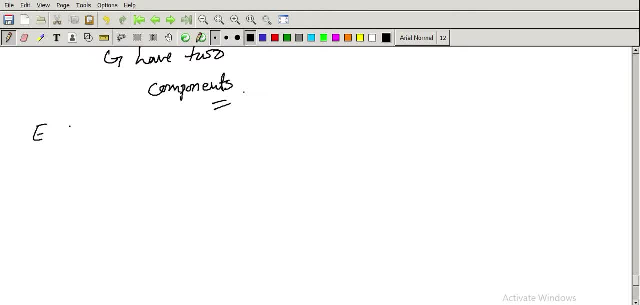 graph right, Euler graph, or Euler path, or Hamiltonian path, right. so let first I write the definition of Euler path, right, because in exams they ask you about this, right? so an Euler path in G is a simple path containing every edge of G, right? what is an Euler path? an Euler path, an Euler path in G is a simple path. right is a simple. 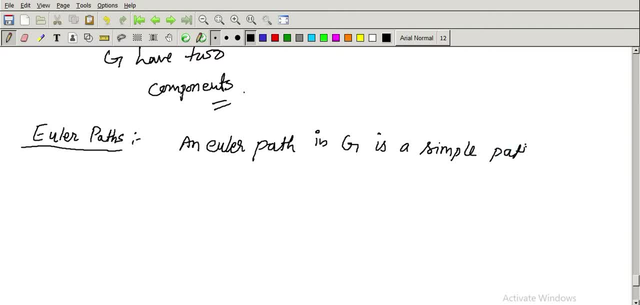 path containing containing, containing every edge of G, right? so this is a simple path, right, as of containing every edge of G, right, ok? so this is the definition for Euler path, right, ok. and what is an Euler circuit? ok, Euler circuit. so you know what is a circuit, if the starting 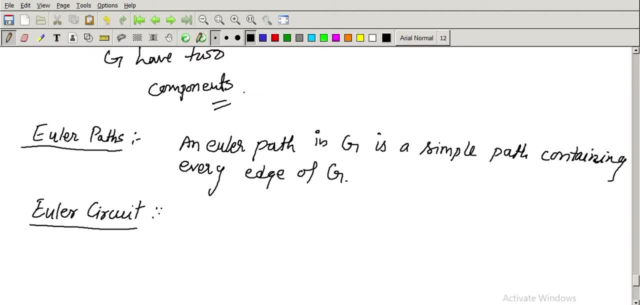 and ending vertex are the same. ok, So it means there is a circuit, right? ok, Euler circuit is an Euler circuit circuit in a graph G. ok, in a graph G it is a simple circuit. it is a simple circuit. it is a simple circuit, right Ok? 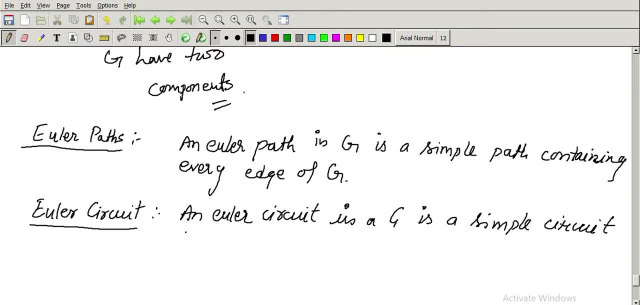 Ok, Ok, and in other words, what is an perhaps a simple circuit? the starting points of the sign of the Euler path are like two parts. Then the sign of the Euler path, Madame, ok, in a graph, two points, right, if the starter point up is going A and the catch point is A for the, the 카�. 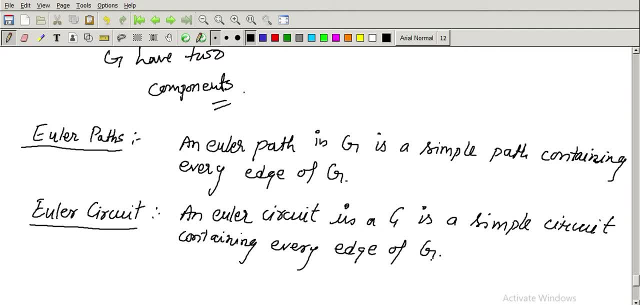 V, k and bottom and so on. so I draw a simple graph for you, right, and we will find that which one has a circuit and which one has an Euler path. okay now, so we have this figure for you, right, just this. and taking this example, right, the example is so okay. so for: 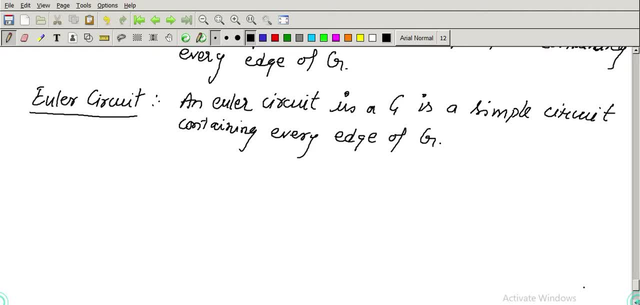 example, this is your example, it. so I have this, these vertices A and B, right, and here I have this. vertices E, right, right, and here we have these numbers are D and C. so this type of graph in which, if there exists in a cycle or not, so in G one, we can see, we 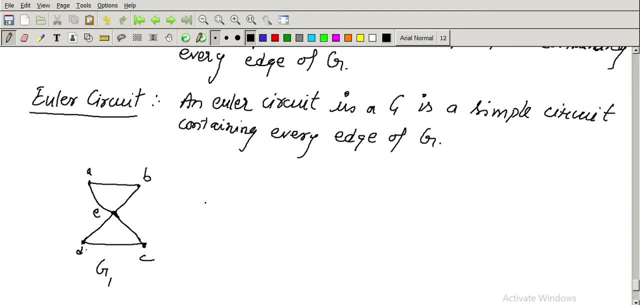 can say easily that if I travel from a, then and I will go to E, right, right, then we go to C, right, A, E, C, then D, then E, then B, then A, okay, right. so A to C, A to E, then E to C, right, then C to D, okay, and then D to E, then E to B. 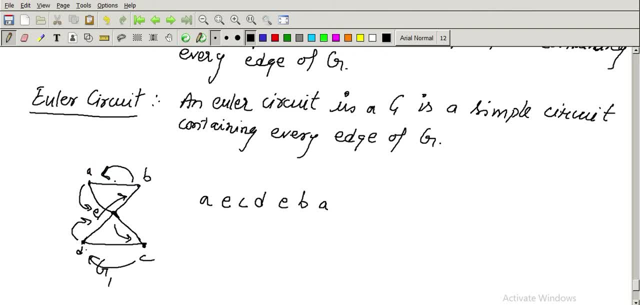 and then D to B, right. so in that case we can find that there is an isle circuit. so in that case we can find that there is an isle circuit because according to the flavor, because according to the flavor circuit definition. that in a graph is a simple. 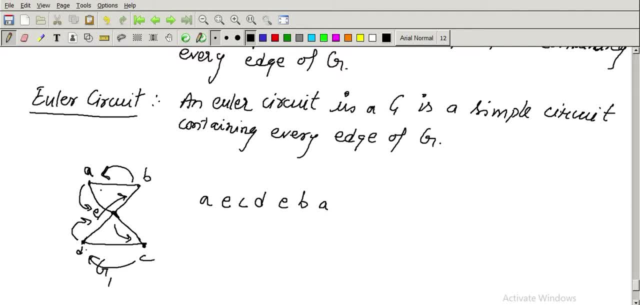 circuit defining every s of C. so they have covered all the s. so in that way we have cover all the edges. so this is a either some great example for einesuc example for either some great example for either some okay, and again they say they're. however, is that from this? how does Hello circuit, depending on what type of 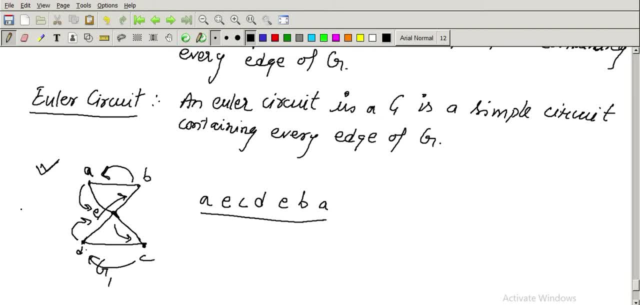 find another circuit. I look path. so you must keep it in mind that the basic difference between the is a circuit and between the circuit and path. so first of all, these two definitions must be clear. so I just told you in the starting of this video video that what is a path and what is a circuit? right, okay, now take 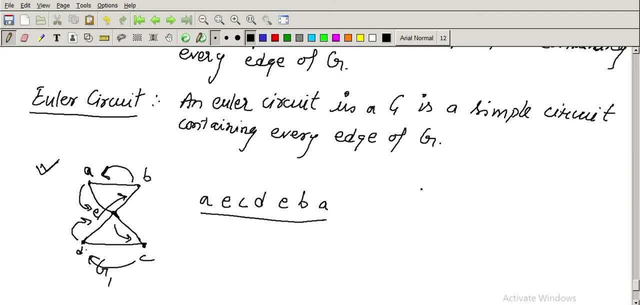 an another example. the example is: this is a graph right, and do remember these definitions of either path and circuit, because they are going to ask in your exam, in your exam. and okay, yes, so here we have this, this graph right. so we have a right a, B. 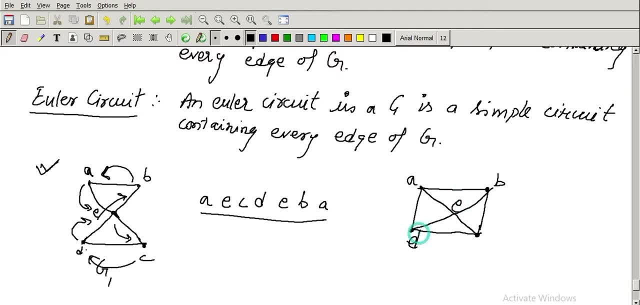 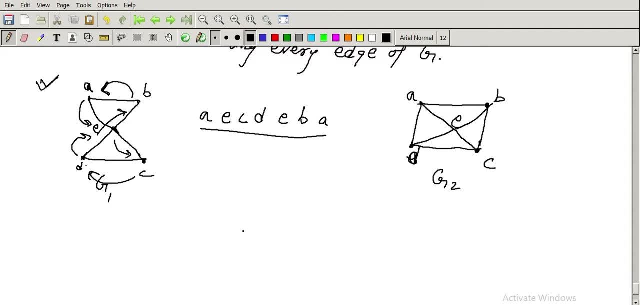 also E, D and C, right? okay, this is your graph. so let's say, this is g2, right? so in g2 graph, taken in g2 graph, we don't have an either circuit, because if I start from a, I go to B, then I go to E, then I go to C, then I go D, then 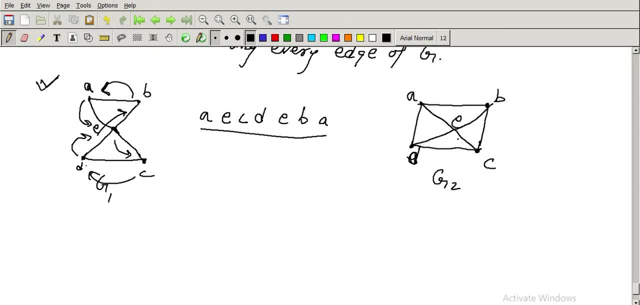 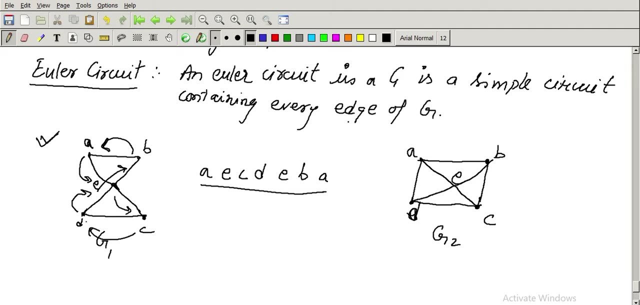 A. so in any way- right, in any ways- it's not possible that we cover the all edges, because because in the definition they say: say that an Euler circuit in a G is a simple circuit containing every edge of G. so if you start from here, you will, you will come back here, but will not cover the entire, all the edges in a. 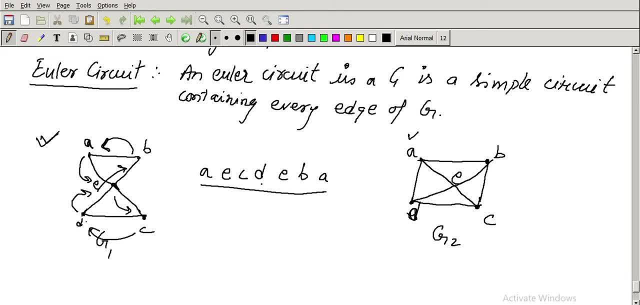 graph, so right. so that's why G2 has not an Euler circuit, right. so this is the example for Euler circuit and right Euler circuit, and because in this graph it has an Euler circuit, right, but this graph is example of not having an Euler circuit, so please keep in. 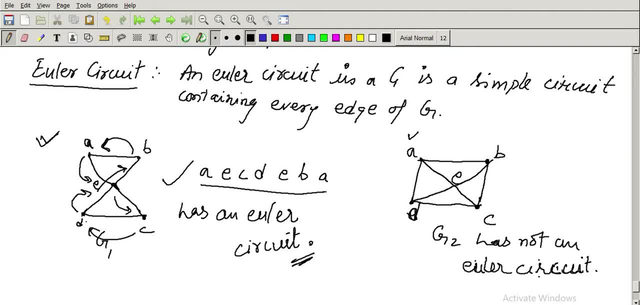 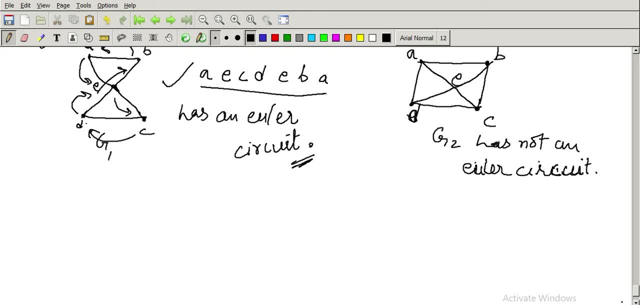 mind the difference. okay, now we move to another right, another concepts. so path is very simple. if you find a path and it it is very, very simple, right? okay, now I like this For the example, for the example, for for Euler pathway, so that you can better understand the concept of Euler path. and then I move to the Hamiltonian. 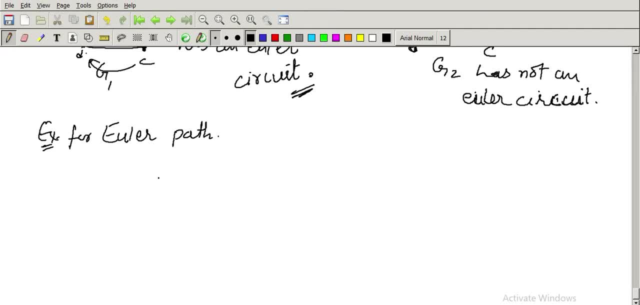 path and circuit, right so? so let me draw a very, very graph for it. right? so now is, this is your graph- which is G2, Euler and Z, which is D1.. Right, so, if F is the final inner orbit, which is like a slight curve, you can draw on each predictor from here. let me draw an but for Euler path, for G to 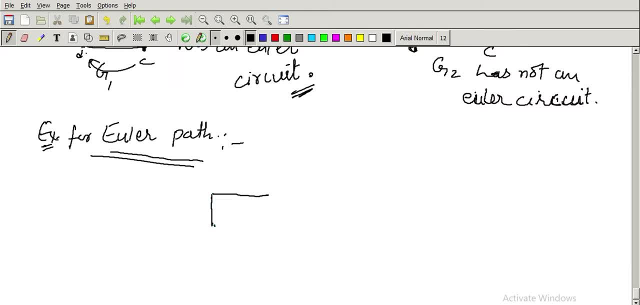 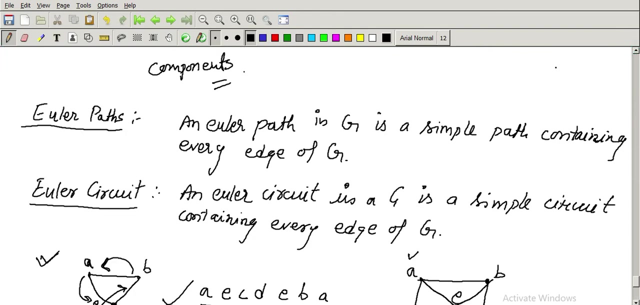 your graph. ok, this is your graph. I have A, B, C, D and E. ok, now you see here that it has an either path. so first of all, for a graph to have an either path, it must be, it must cover all the right, what, all the edges of C, another path in Jesus. 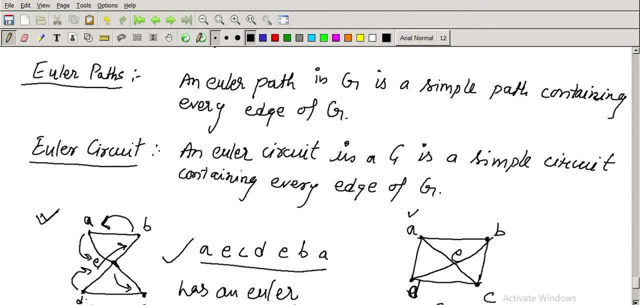 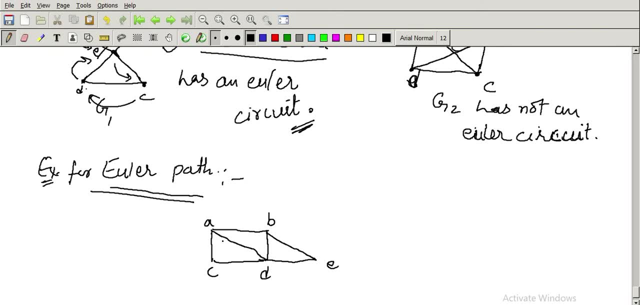 improper containing every s of G. so is, is that possible? in that example, we, we, we are covering all the edges. so so let's find, ok, let's find. if we can find a path, right, so for a start, from a right a to C to D, right, ok, then then be right. ok, can can we go right? we can go. 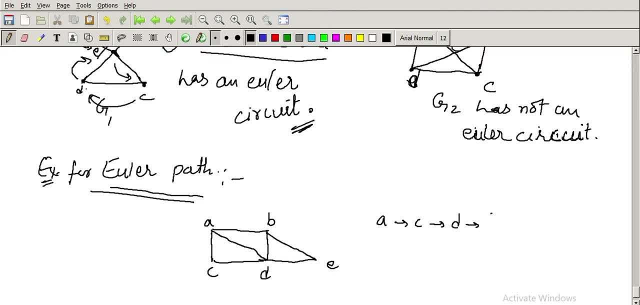 right: a, a, C, then D, or then. then we let's say then he, ok, so we have cover these, this vertex, this vertex- sorry, this is this as an- this is ok, now we go back to this, right he, and then be right, then, then I have covered this right then today, and okay, then this one might be 2d. 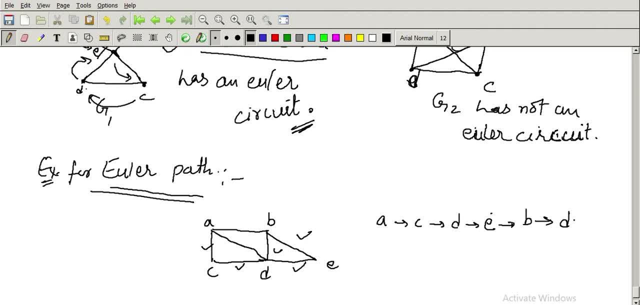 and then right and then B. so in that way, right, we have covered all the edges in this graph, right? so this, this, this graph that says g3, contains a, either path, right, either path. so does it contain a circuit? either circuit or not. because, and in either circuit, there it must cover all the. 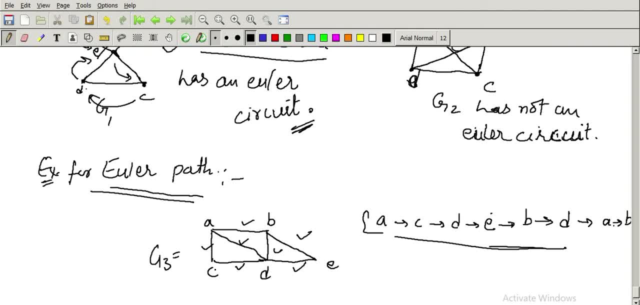 all the edges which it has already covered in this example, but it comes back to the same vertex, or same starting vertex means so what is path? path means you have to cover all the edges, cover all the edges, but it's not necessary, but it's not necessary. 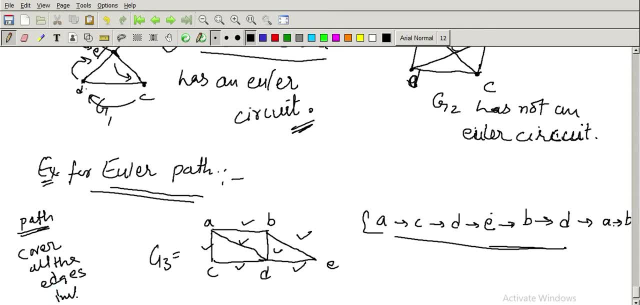 but it's not necessary that the initial vertex, initial will be your, will be your end. so you start. you start from that that vertex and you cover all the edges and come back to this vertex. it becomes a circuit. right, it becomes a circuit. but if you cover all the edges, okay, all the edges. 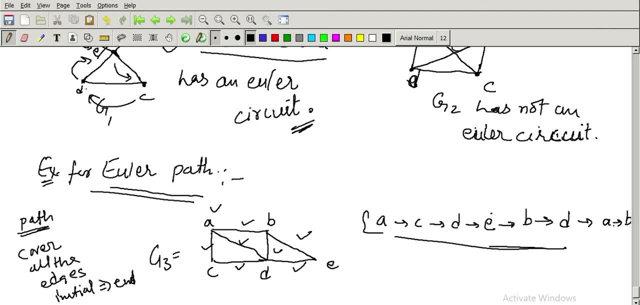 but you don't reach to this. so this is your path, right, this is your path. so in path its not necessary initial line, but in a circuit the definition is the same. like you have to cover all the edges, all the edges, but your starting vertex and ending vertex, you know the starting and ending will be same, right? so that's why that's. 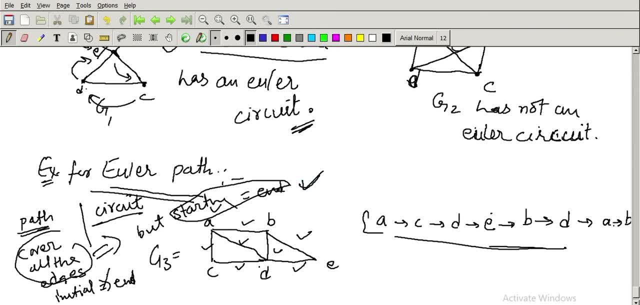 why we are saying that it has path. it has a path because of this example. here you are saying that it has a path, so that the path is much bigger, so that the very starting from green, for example. this is here you have an input, here you will see that on edge you can. 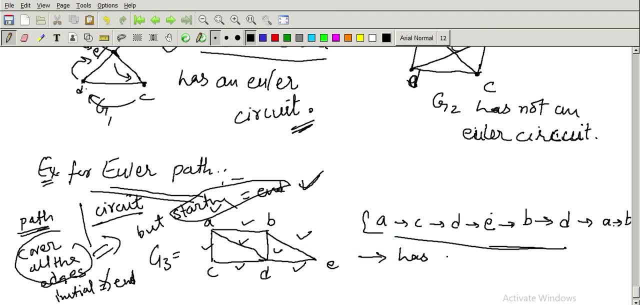 see that the logic behind the states, when you don't leave this feature, will be related to the: a path has a path, but not circuit. but not circuit because, four-circuit, there is a necessary or there is a necessary condition. okay, that it must be that when 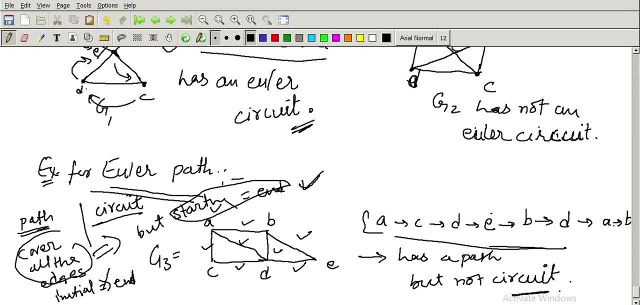 you, when you start from a vertex, you must end by covering all the edges to that particular vertex. so it's not the case here, right? so I think this concept is very much clear to all of you, right? okay, now we go back to the Hamiltonian right Hamiltonian circuit and path. okay, so first of all, we must know that. what? 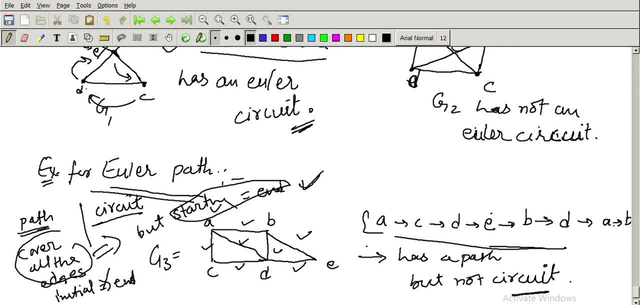 is in Hamiltonian path and Hamilton circuit. but before that there is a right. there are two theorems that they might be asked in your exams, right, based on this concept of Euler path and circuit. so I discussed with the this, these two terms right. so first, 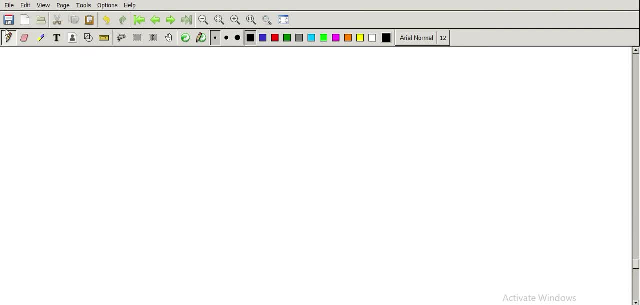 theorem is your. the theorem one is the first. theorem is your. the theorem one is the first. theorem is your. the theorem one is the first theorem is your. one is a connected, the connected multi graph. so you know, you know that what is a multi graph? if you don't know, please was the. 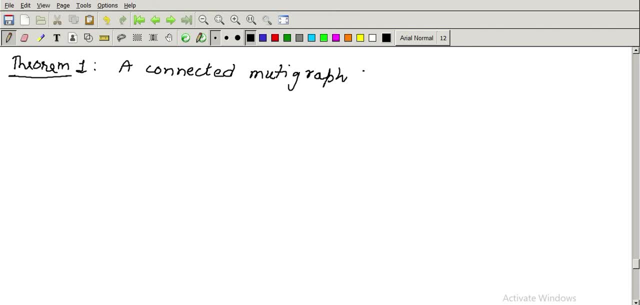 first videos in the series of discrete mathematics. they connected multi graph with at least two vertices, with at least two. what this is? and lautr circuit, right alert circuit, and you know what is international. okay, if and only if, if and only if, if and only if if. 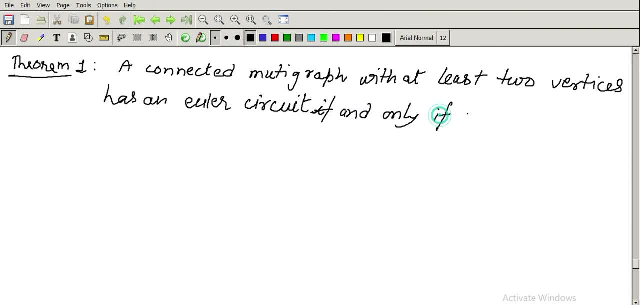 if, if and only if, each of its work vertices, each of its vertices, has even degree, has even degree, right? okay, so this theorem says that a connected multi graph with at least two vertices has an Euler circuit if, and only if, each of its vertices has even degree. okay, so what should be the vertex of every vertex? 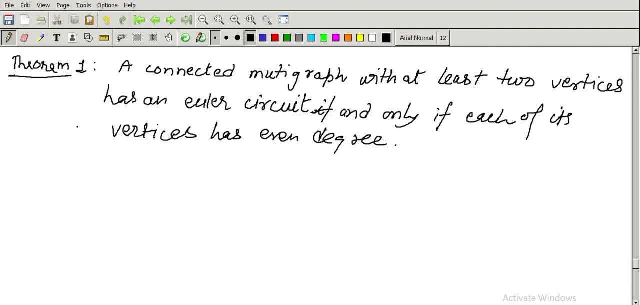 even degree. so so, for a multi graph which has at least two vertices, which has at least two vertices, in that graph there is an Euler circuit and, as it exists, it follows the definition of Euler circuit only if, and only if each of its work vertices has an Euler circuit. 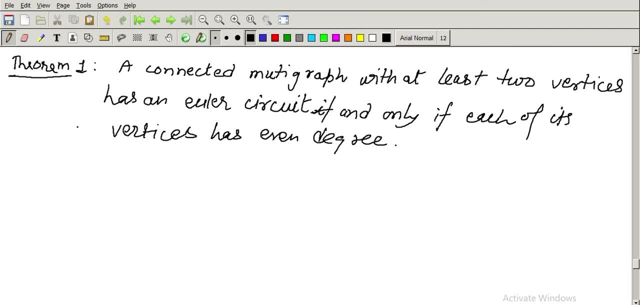 only if each has an Euler circuit, only if each of its work vertices has even degree, right, right, so. so, for example, it. so, for example, for example, we have this Kong Kong-Berg-Britz problem, right, so, okay, so you must remember this, right, so you must remember, you must remember. 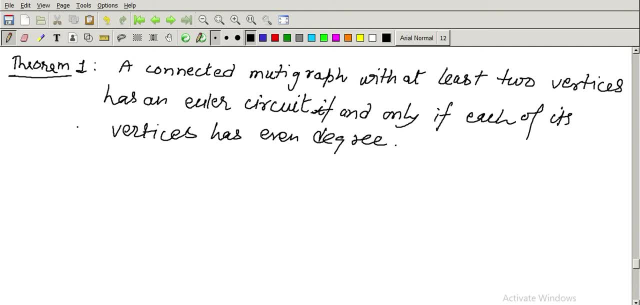 this definition of theorem that what is it right? okay, now the second theorem is- and I will definitely solve some questions based on these theorems- right questions means that I will prove with proof that what are the examples of these, these examples on these two theorems, right? so the second theorem says that a 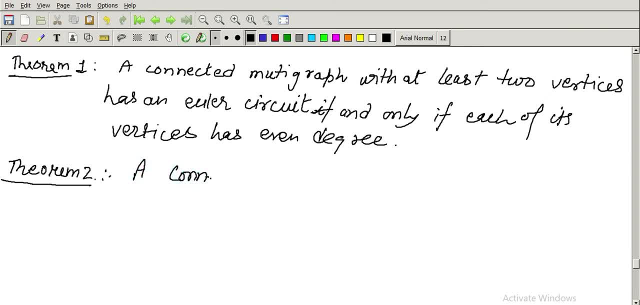 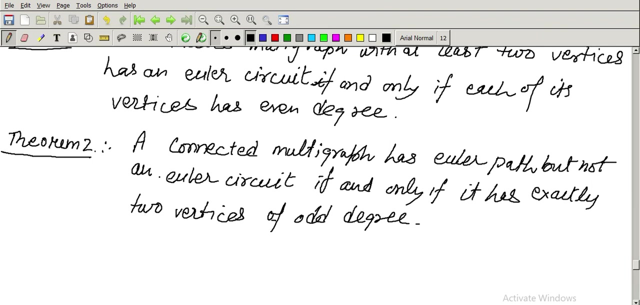 connected multi graph, a connected multi graph, a connected multi graph has an euler path, path, path, but not an euler circuit, right, not an Euler circuit. Euler circuit, Euler circuit, if only, if, if and only if it has exactly two vertices, two vertices of odd-degree right, two vertices of odd-degree right. okay, so here, if I 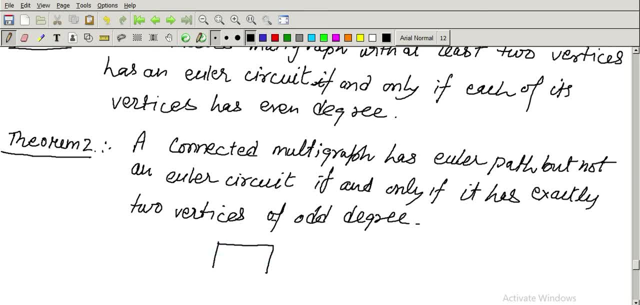 for an example, if I take this simply, this is a graph a, B, C and D. okay, so it has an Euler path, Euler path, Euler path. when I start with this right. so I must be covering all the edges, right. so I go to A to B, right, A to B. 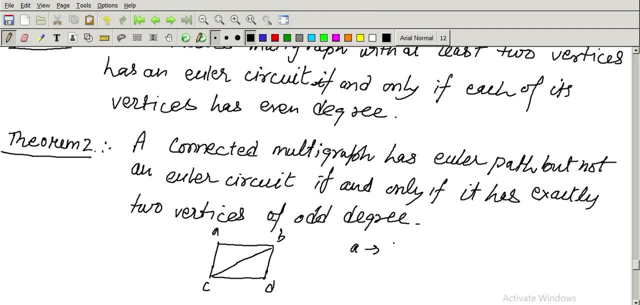 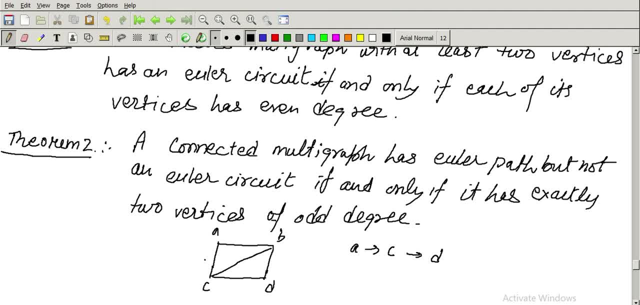 right then. so here you have, you started from A, A to C. you have covered this, right, you have covered this. then you go to B, you record this, you go to this, you code this right, okay, so as is it. it has an Euler path. so in that way, we, we are. 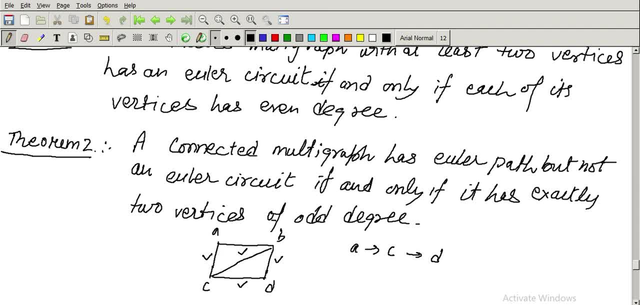 code this, right, so as is it, it has an Euler path, so in that way, we we are not covering this one, so let's find another. okay, not covering this one, so let's find another. okay, let's find another path, another path, another path is your if I start with the D. right, I start with D because I can start from. 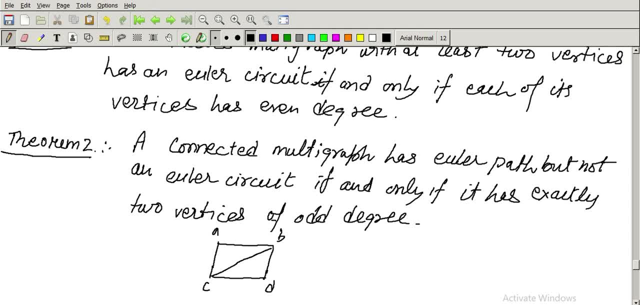 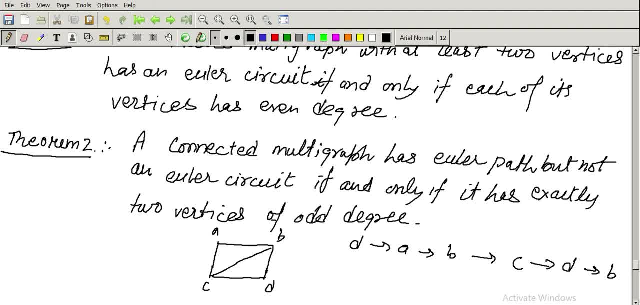 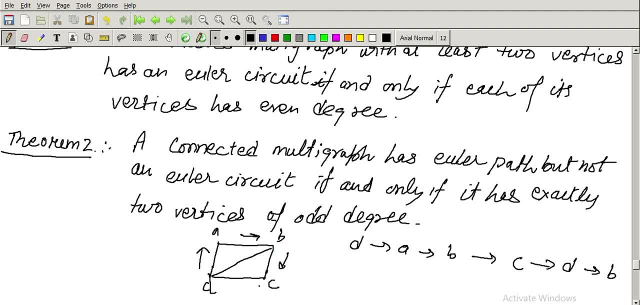 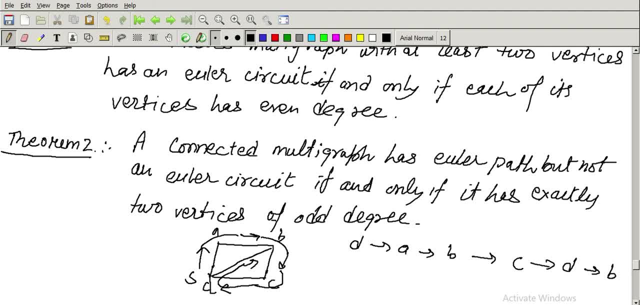 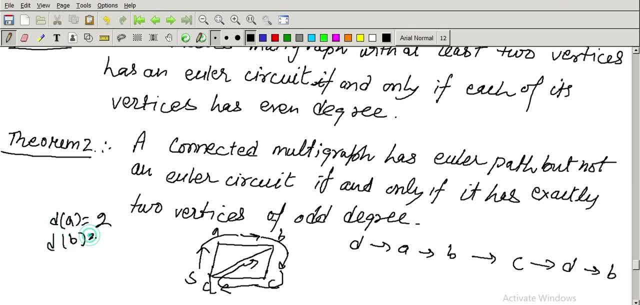 2. degree of B is 3. degree of C is 3, 2- sorry. degree of D is 3. so according to this term, it must have two vertices of all degree. so these are the two vertices: B and D. B and D has all degree because it is 3. 3 is an odd number, so it has two vertices of all degree. 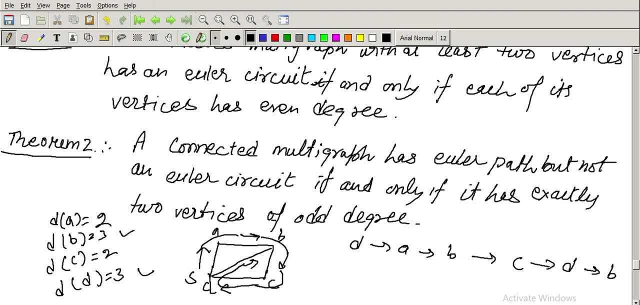 right. so I we can say that when this is the condition, so it has an Euler path, so there exist an Euler path in that case when two vertices are of odd degree. okay, so so these are the two theorems and on the concept of this Euler path and circuits, I hope that it. 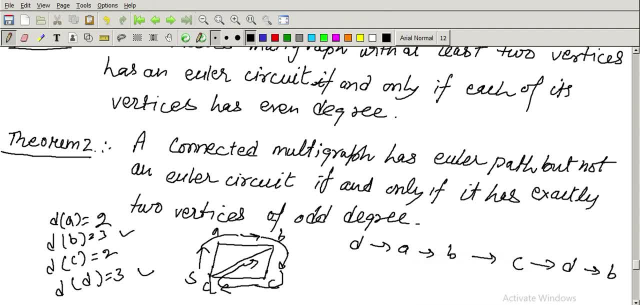 will be helpful for you, right? so thank you.